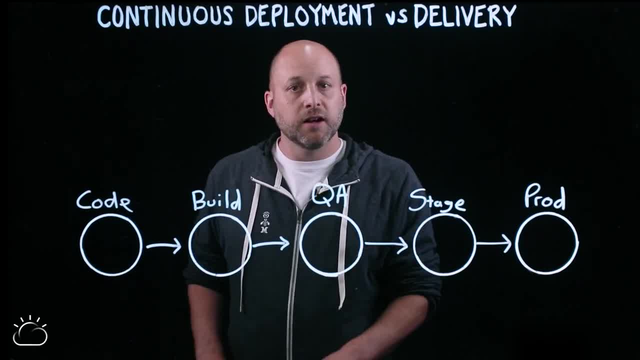 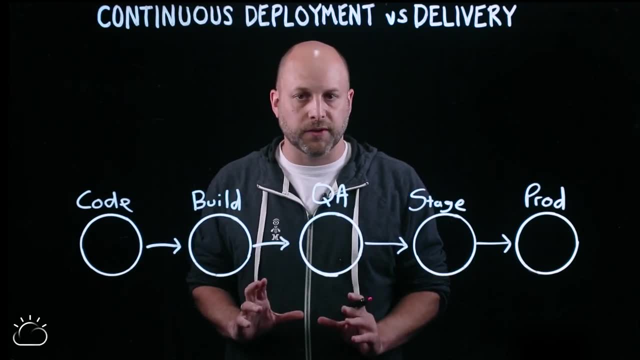 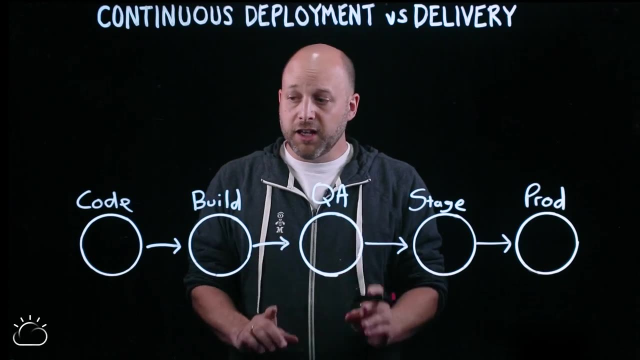 test environment, So they brought these things together. But thousands of tests, really robust testing suite that ran across a large number of servers so that you could run thousands and thousands of tests in a short period of time and know that your new code was probably pretty good because you'd run these robust set. 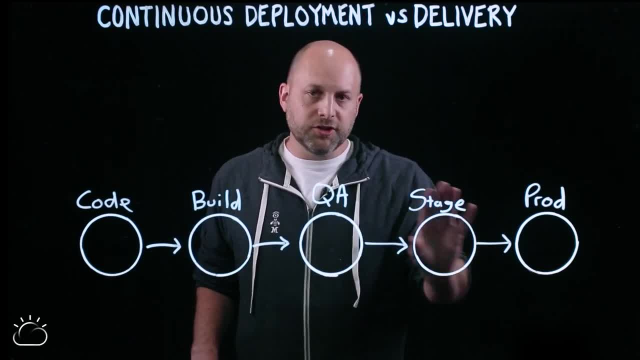 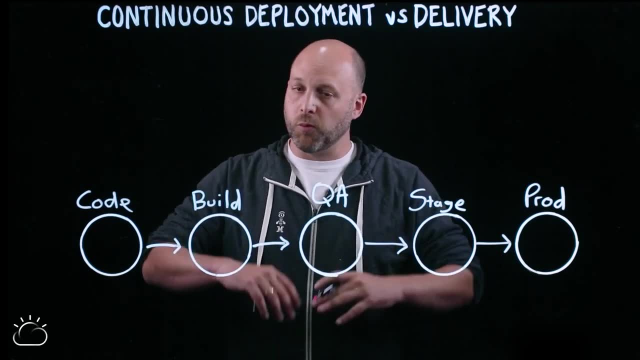 of tests that you could depend on, And because you believed in your testing, you could put that out into production. Now, this was a consumer-facing app. It wasn't taking credit cards, And so you could just put that out to 2% of your 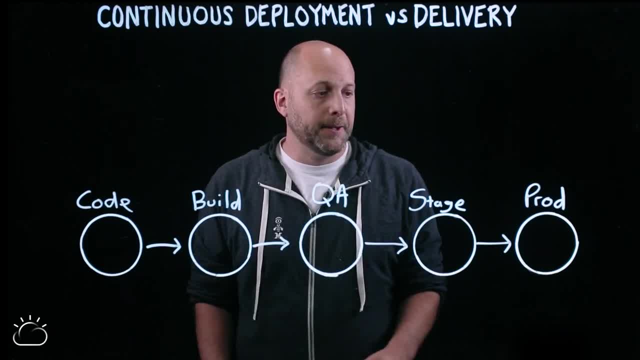 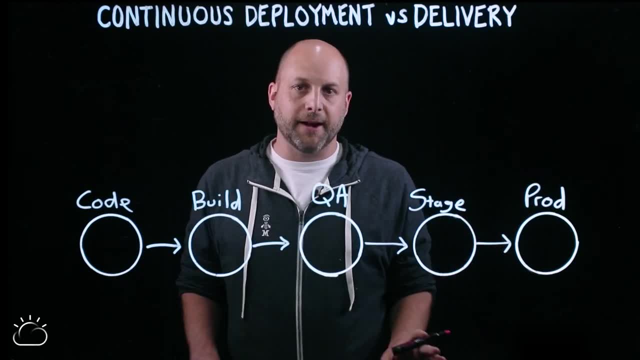 users, or 5% of users, do what's known as a canary deployment and make sure that the servers weren't falling over, that people were still interacting with the app as they should. So you had a robust testing suite, and then you were also. 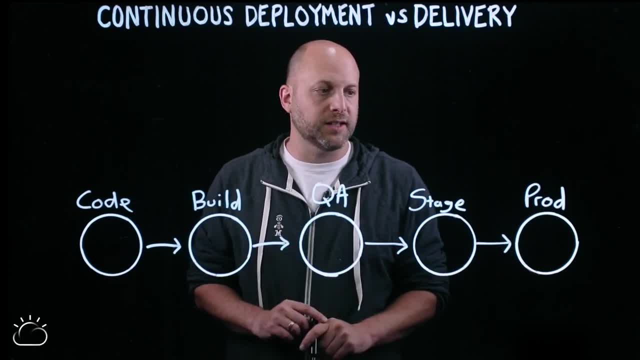 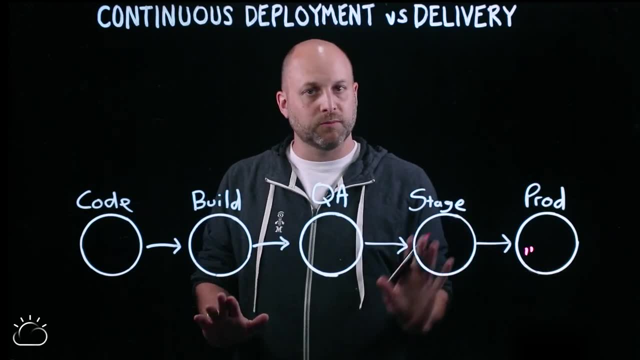 testing in production. right, You were monitoring really robustly and if things were going badly out here in production, if, like, two of your servers keeled over, okay, you're gonna pull that change out of the load balancer you have. 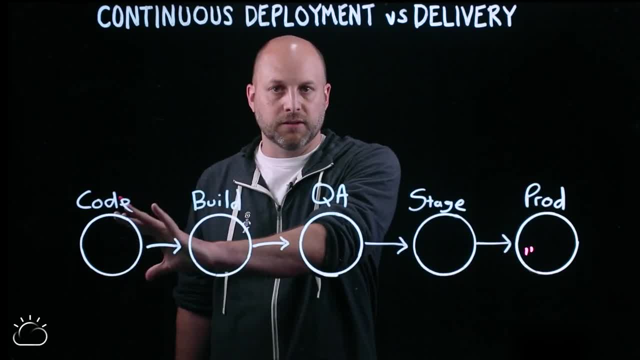 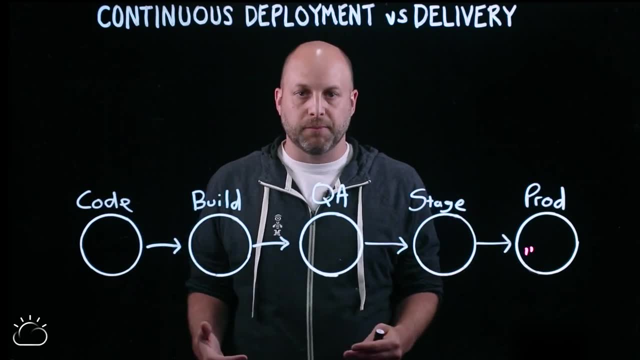 the rest of your servers working, fine. you can go back and fix it in code. It'll go right back out the door real quick, Nice. So this is really an extreme approach. Someone writes code, it ends up in production. no one else touches it. 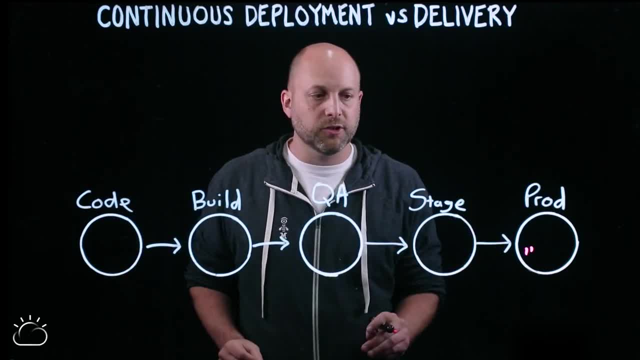 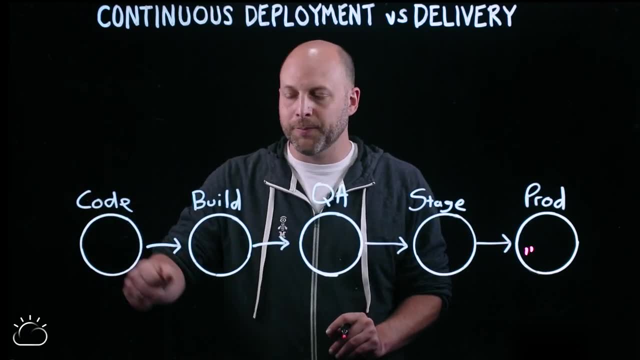 Where you have a little bit of regulatory approval and you need two eyes on anything before it gets to production. back here in code review, back here in code you can do a code review and another developer can provide that check And then the testing provides you with. 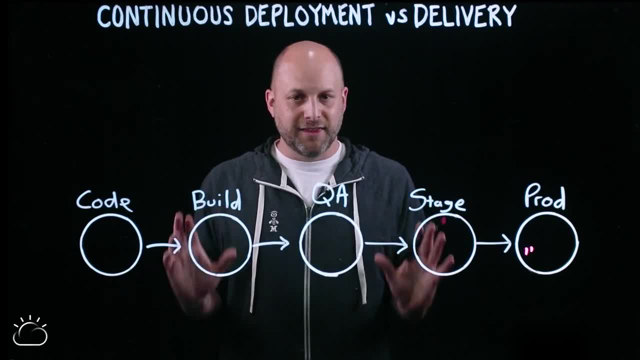 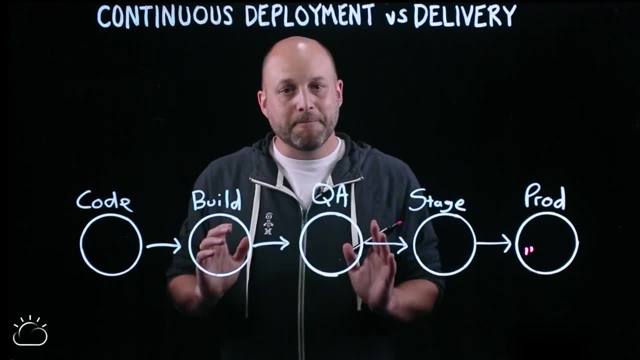 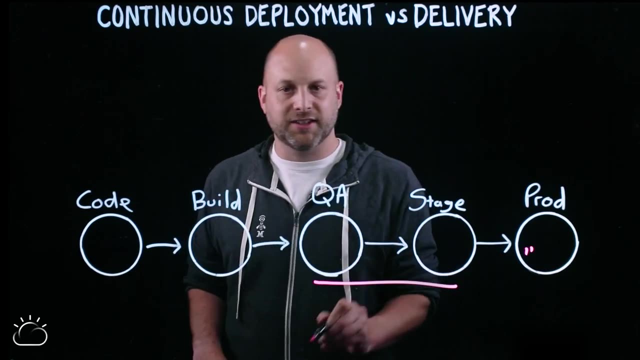 another safety net. Now, this approach, this continuous deployment, continuous deployment to production, is really what it means. That's still extreme and something a lot of organizations both don't have the testing for, nor do they have either the kind of stomach or the